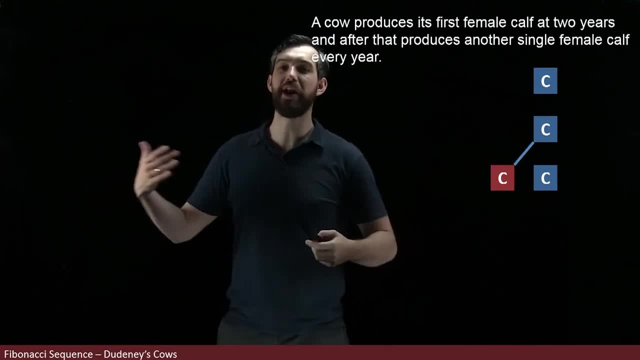 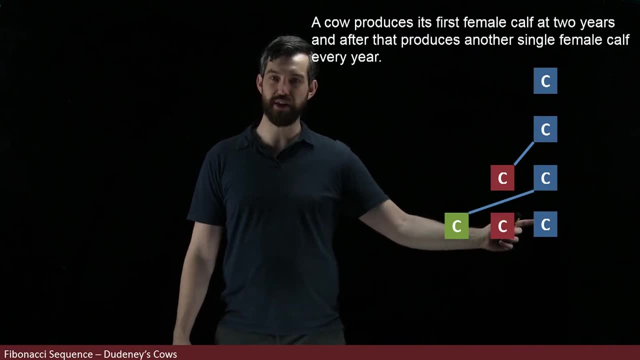 cows, but the original one still does. they're making one every single year, So I believe I should have three down at this level: the two that I started with, the original and the new cow, and then we get one more one that is being born. so I 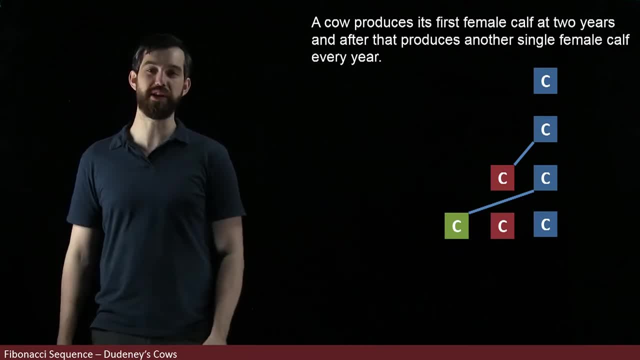 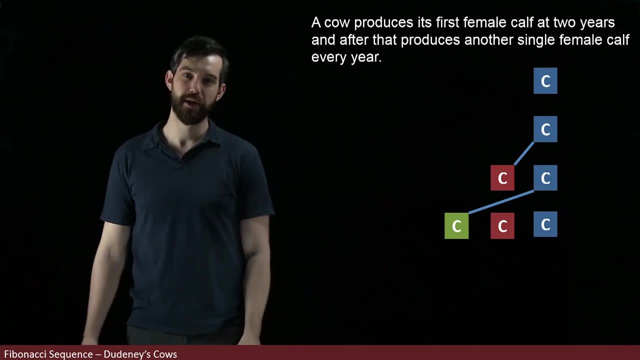 have a total of three. Okay, let's go one more year into the future. Well, all three of these that I have, we know that they're gonna still be there, so we'll for sure have three. The blue original cow that's gonna produce one. 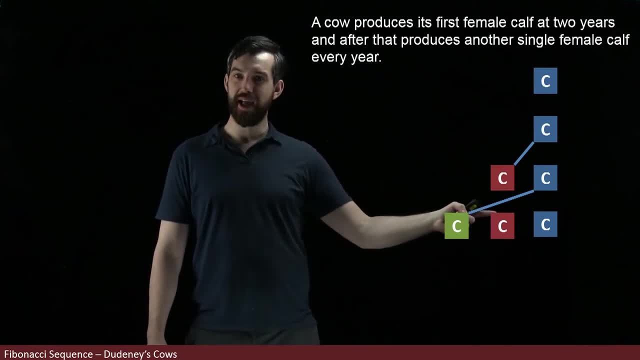 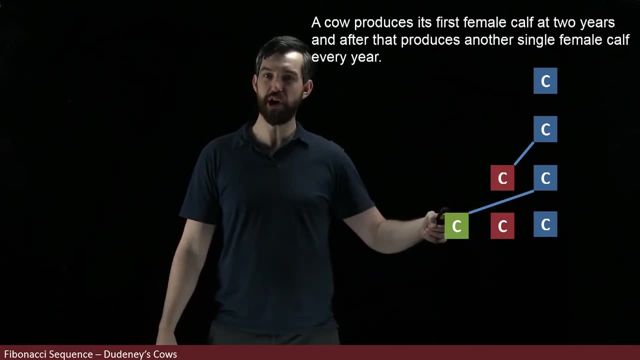 it's making one every single year, but but now the red cow is two years old and is old enough, and so she is also making new cows, So we're gonna have the three that we started with, plus the two from the prior level are gonna make two. 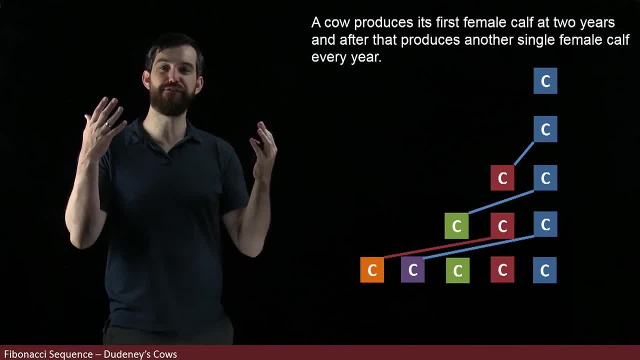 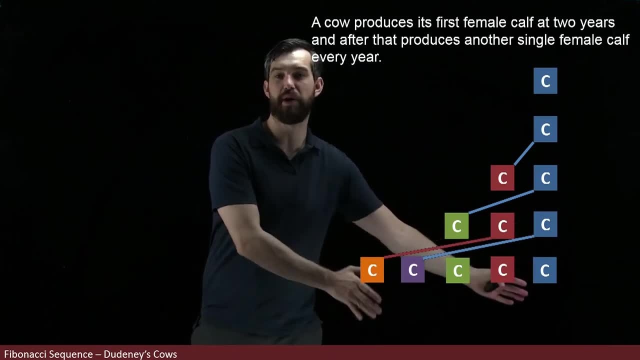 additional ones, and so I'm gonna a grand total of five. Then I hope we see how the patterns turn to go Okay, in the next year. we have these five. all five of them are gonna live, But it's not the five that's gonna be. 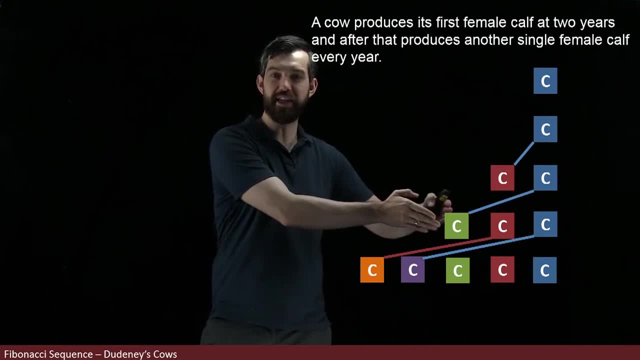 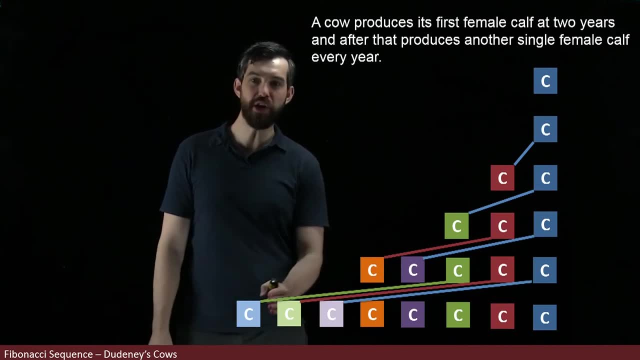 able to reproduce. It's the previous step. these three that we have here, they are now gonna all be old enough to reproduce, and so we're gonna have three NOW new ones. those are going to be reproduced by the three that were at this stage, plus the five that 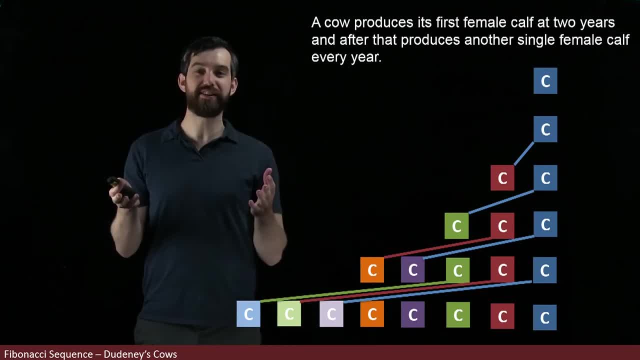 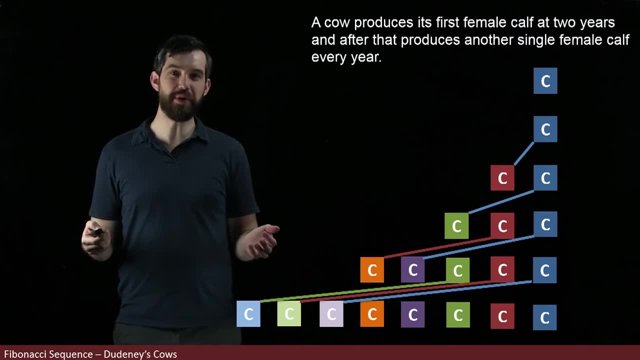 we had. So then if I let f of say three denote how many cows I have in the third year, then we can count them like this: There's one cow in the first year, one cow in the second year, two, three. 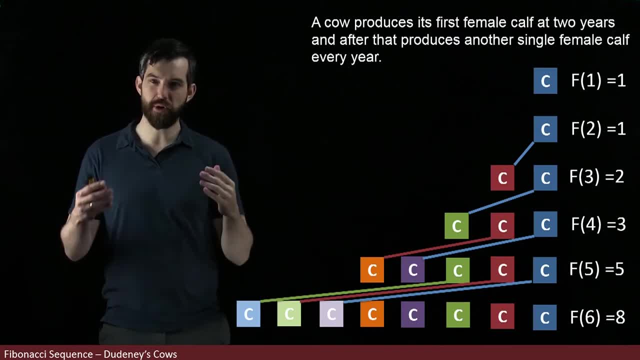 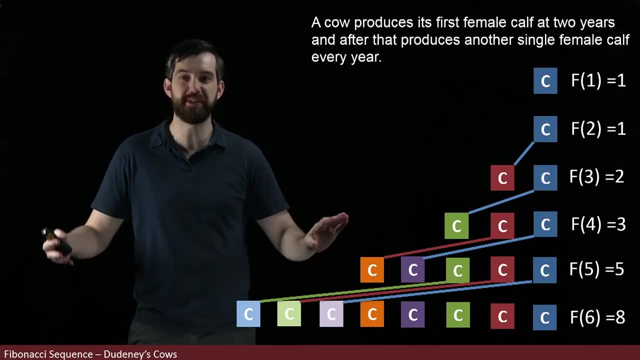 five and eight going forward. Now. the key insight that I want you to notice here is that let's focus for the moment on the fifth year. I'm trying to make the fifth year, which happens to have five cows. It was going to be the sum of two things: The sum of the amount of cows in the fourth year. 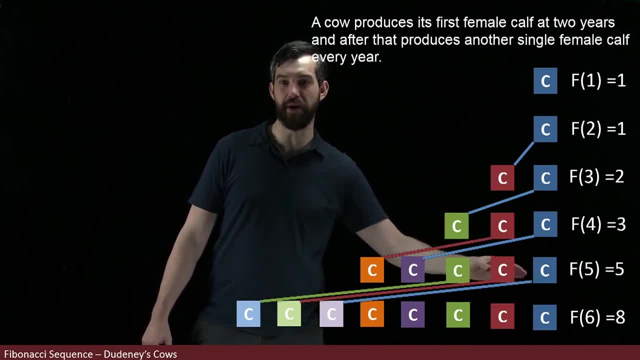 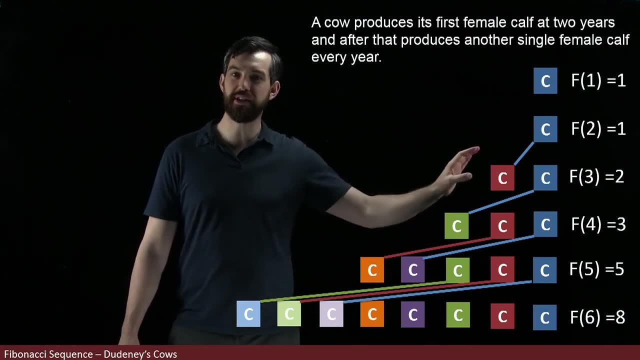 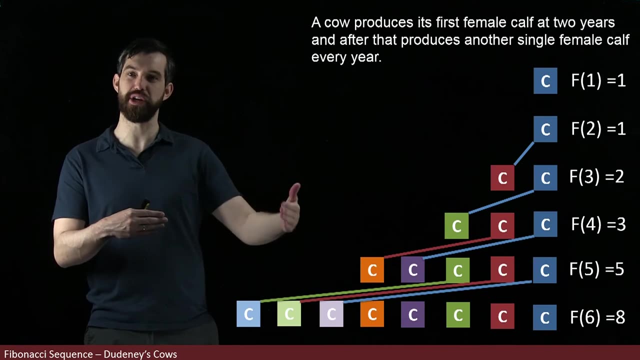 because all of those cows they just survive and they carry on. So it's the sum of the things in the fourth year plus the amount of cows in the third year, because it's the third year cows they're able to reproduce and make these extra new ones in the fifth year because of that two-year.